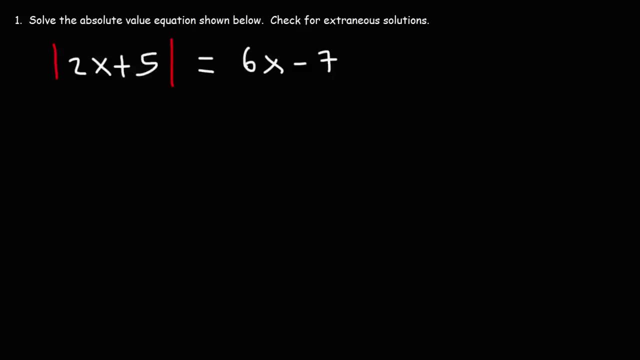 Go ahead and solve this equation and then check your solutions to see if any of them are extraneous. The extraneous solution that we're looking for is the solution that doesn't work in the original equation. That's the one we need to throw out. 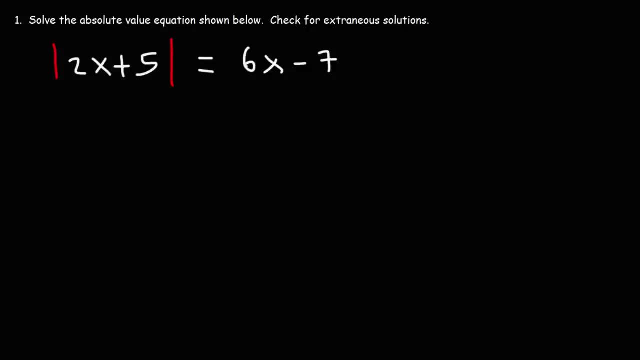 So let's go ahead and begin. In order to solve this absolute value equation, we need to write two equations. When we open up, When we open up the absolute value symbol, we're going to set what's inside equal to the positive value of what's on the outside. 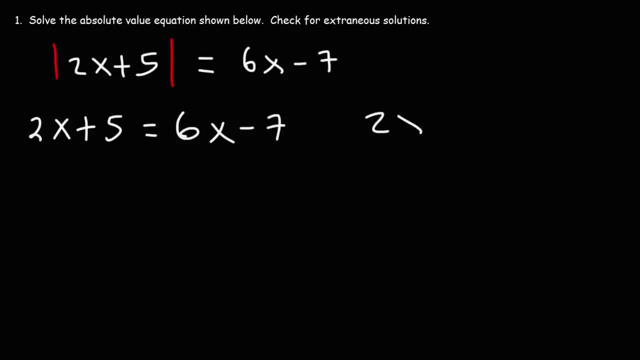 That is 6x minus 7.. And we're also going to set what's inside of here equal to the negative value of what's on the right side of the equation, In this case negative 6x minus 7.. So let's start with the equation on the left. 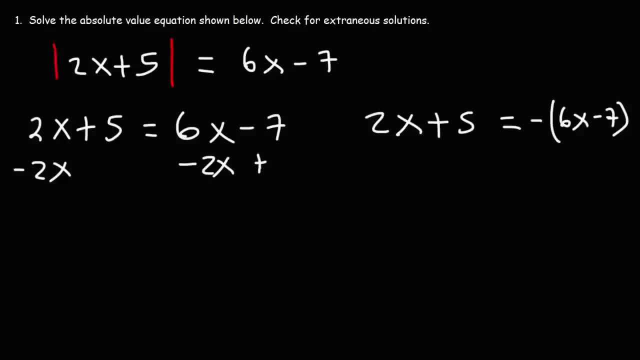 Let's subtract both sides by 2x and let's add 7 to both sides. Our goal is to isolate x in order to solve the equation. So 2x and negative 2x will cancel, and the same is true for negative 7 and positive 7.. 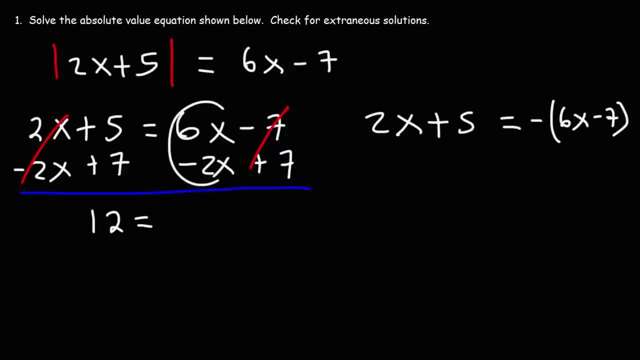 5 plus 7 is 12.. 6x minus 2x, 2x is 4x. Now, to get x by itself, we need to divide both sides by 4.. 4 over 4 is 1, giving us x. 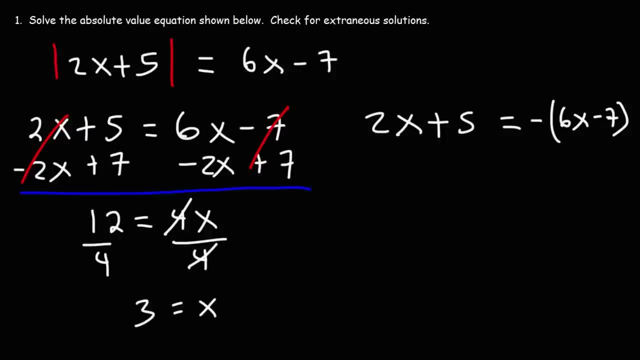 And on the left we have 12 divided by 4, which is 3.. So this is one potential solution. x is equal to 3.. Now let's move on to the equation on the right side. The first thing we're going to do is distribute the negative sign to 6x and negative 7.. 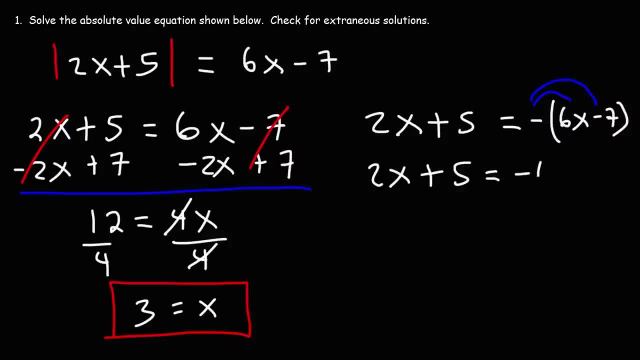 So we're going to have: 2x plus 5 is equal to negative 6x, and then negative times negative 7.. You can see it as negative 1 times negative 7. That's going to be positive 7.. Now let's subtract both sides by 5.. 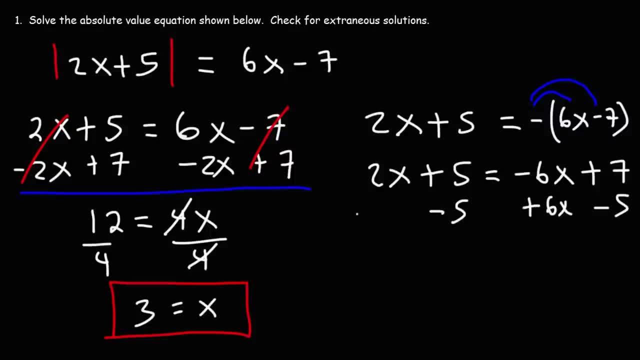 And let's add 6x to both sides. So we're going to have: 2x plus 5 is equal to negative 6x and then negative 7.. And let's add 6x to both sides. 2 will cancel, and the same is true for those two. 2x plus 6x, that's going to be 8x. 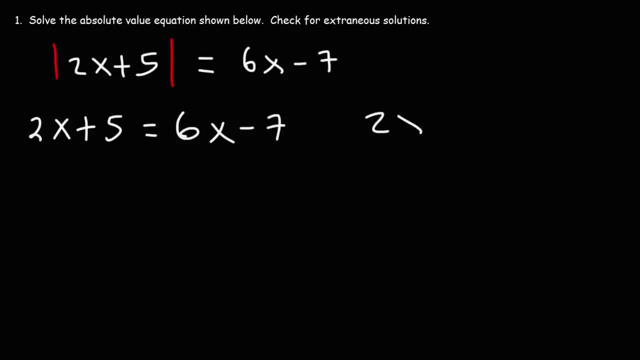 That is 6x minus 7.. And we're also going to set what's inside of here equal to the negative value of what's on the right side of the equation, In this case negative 6x minus 7.. So let's start with the equation on the left. 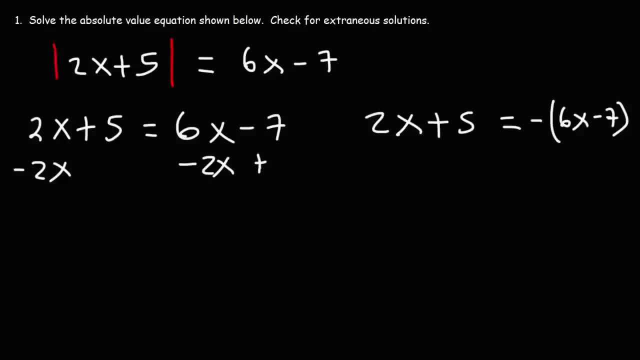 Let's subtract both sides by 2x and let's add 7 to both sides. Our goal is to isolate x in order to solve the equation. So 2x and negative 2x will cancel, and the same is true for negative 7 and positive 7.. 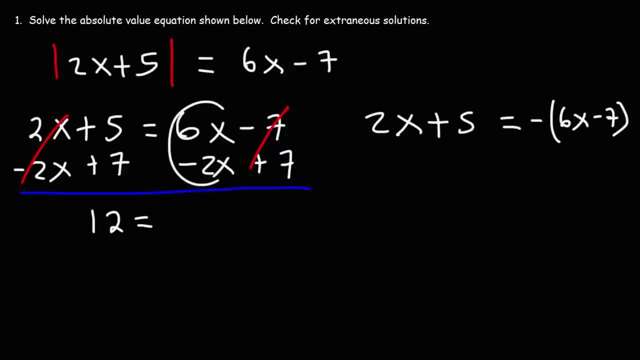 5 plus 7 is 12.. 6x minus 2x, 2x is 4x. Now, to get x by itself, we need to divide both sides by 4.. 4 over 4 is 1, giving us x. 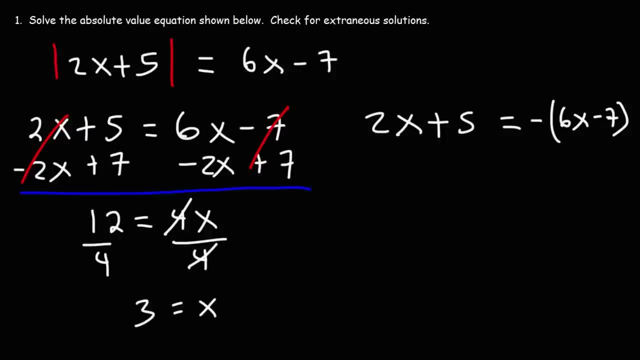 And on the left we have 12 divided by 4, which is 3.. So this is one potential solution. x is equal to 3.. Now let's move on to the equation on the right side. The first thing we're going to do is distribute the negative sign to 6x and negative 7.. 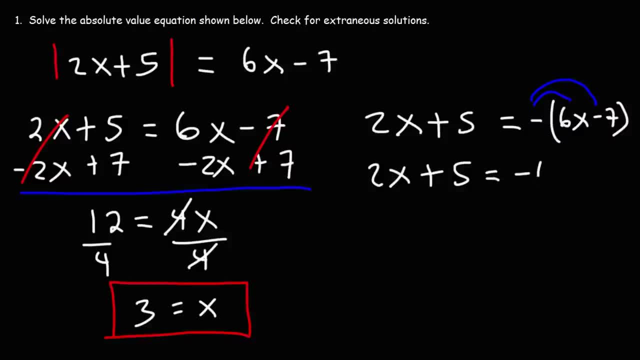 So we're going to have: 2x plus 5 is equal to negative 6x, and then negative times negative 7.. You can see it as negative 1 times negative 7. That's going to be positive 7.. Now let's subtract both sides by 5.. 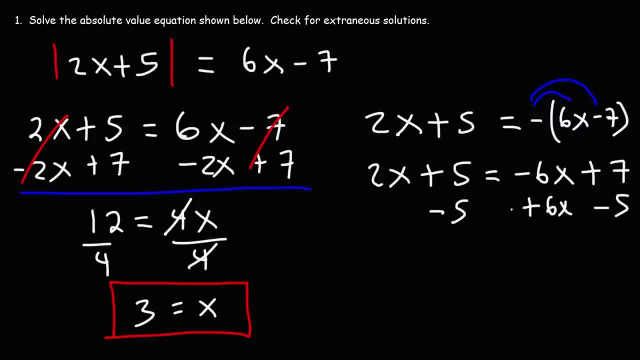 And let's add 6x to both sides. Subtract 2x, 5.. Subtract 6x. So these two will cancel, and the same is true for those two: 2x plus 6x, that's going to be 8x. 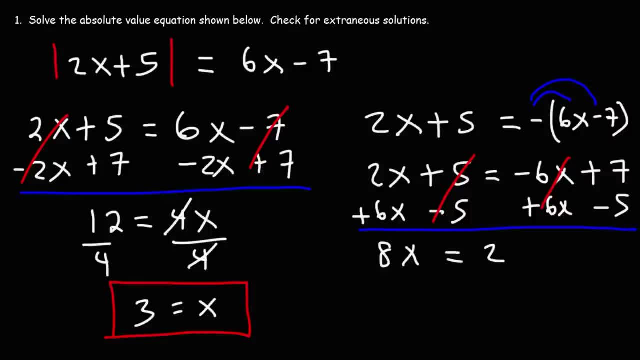 And then positive 7 plus negative 5,, that's positive 2.. So to separate 8 from x we need to divide both sides by 8.. So x is 2 over 8, and 2 over 8, we can reduce that. 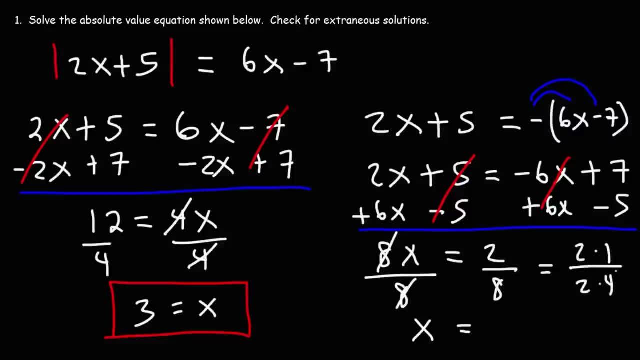 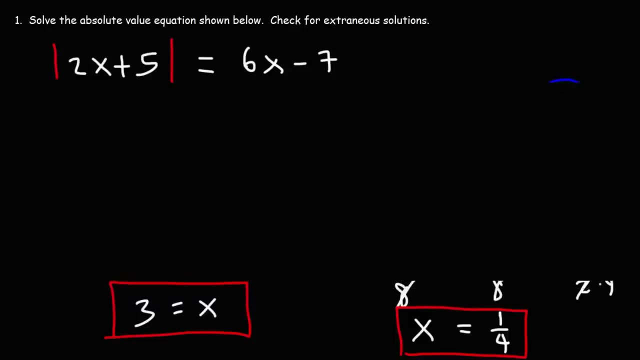 This is 2 times 1, and 8 is 2 times 4.. Now, canceling out a 2,, we get 1 over 4.. So these are the two potential solutions. Now let's see if they work for the original equation. 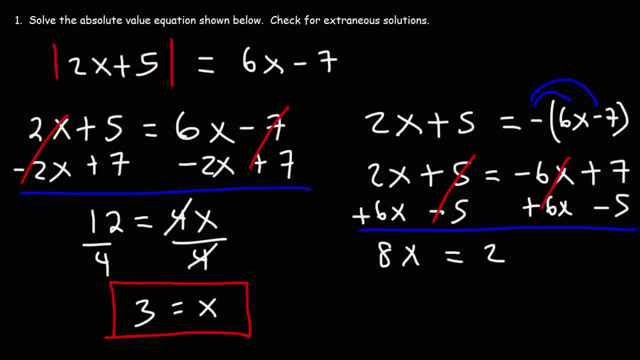 And then positive 7 plus negative 5,, that's positive 2.. So to separate 8 from x, we need to divide both sides by 8.. So x is 2 over 8, and 2 over 8, we can reduce that This is 2 times 1, and 8 is 2 times 4.. 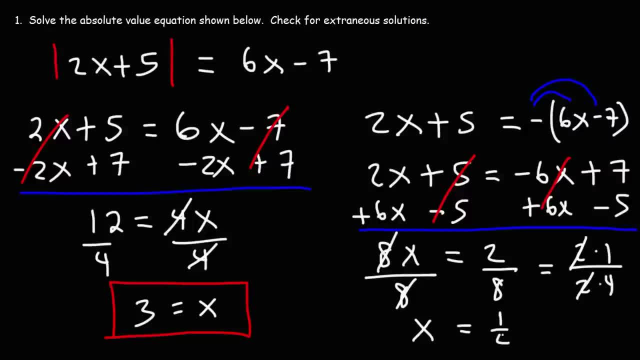 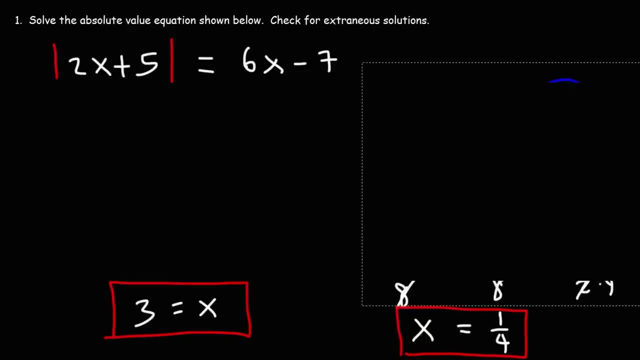 Now canceling out a 2, we get 1 over 4.. So these are the two potential solutions. Now let's see if they work for the original equation. So let's start by plugging in 3 into the equation. 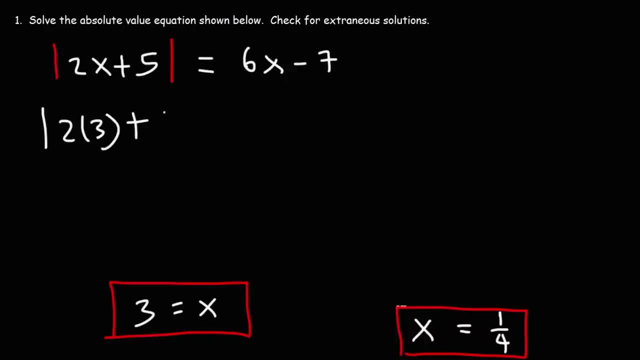 So, replacing x with 3, we have 2 times 3x 3 plus 5.. On the right, we have 6 times 3 minus 7.. 2 times 3 is 6.. 6 times 3 is 18.. 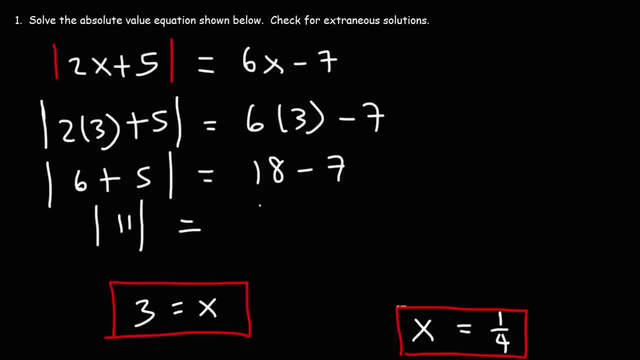 6 plus 5 is 11.. 18 minus 7 is 11.. The absolute value of 11 is 11.. So we have: 11 is equal to 11, and that works. So x equals 3 is a true solution. 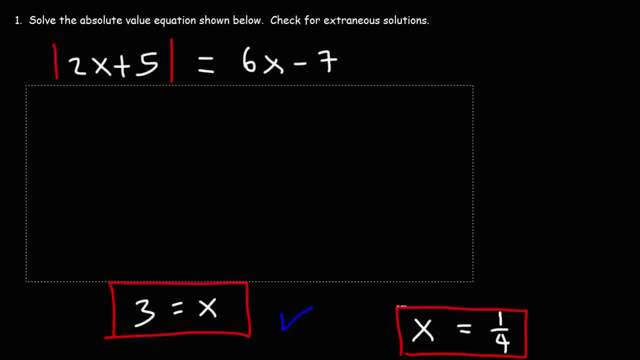 So we're going to convert the solution to the original absolute value equation. Now let's check the other solution: 1 over 4.. Let's see if this works. So 2 times 1, fourth, 2 times 1 is 2, so this becomes 2 over 4.. 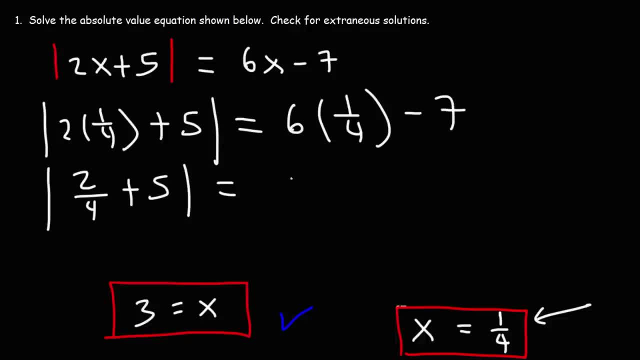 6. 6. times 1, 4th, we can write that as 6 over 4.. Now let's simplify the fraction: 2 over 4, that's 1 half if you divide both numbers by 2.. And 6 over 4,: 6 is 3 times 2, 4 is 2. 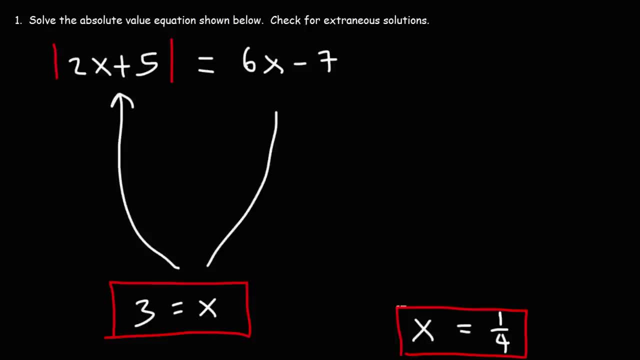 So let's start by plugging in 3 into the equation, So replacing x with 3, we have 2 times 3.. 3 plus 5.. On the right, we have 6 times 3 minus 7.. 2 times 3 is 6.. 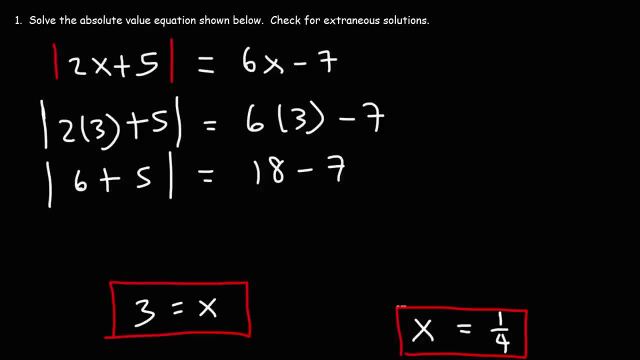 6 times 3 is 18.. 6 plus 5 is 11.. 18 minus 7 is 11.. The absolute value of 11 is 11.. So we have: 11 is equal to 11, and that works. 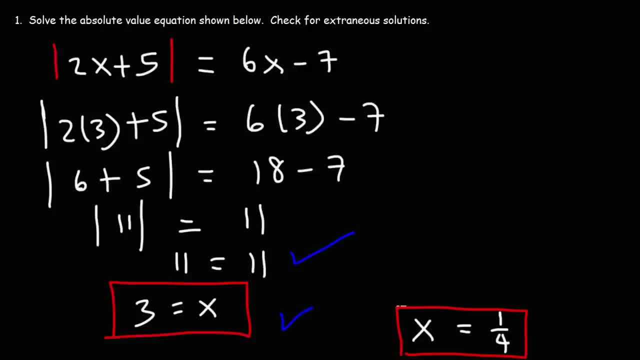 So x equals 3 is a true solution. So x equals 3 is a true solution to the original absolute value equation. Now let's check the other solution, 1 over 4.. Let's see if this works. So 2 times 1. fourth, 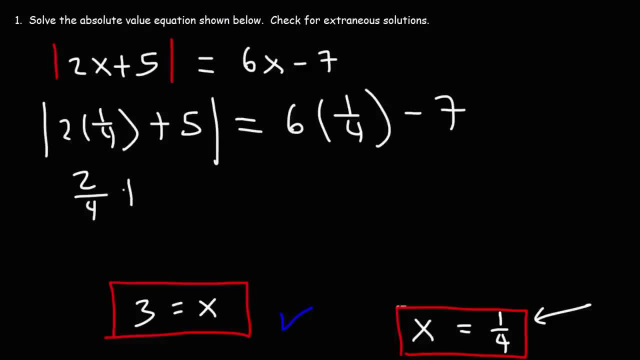 2 times 1 is 2, so this becomes 2 over 4.. 2 over 4. 6. 6 times 1. fourth, We can write that as 6 over 4.. Now let's simplify the fraction. 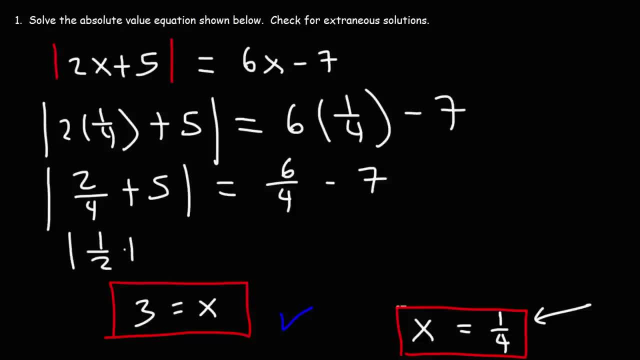 2 over 4, that's 1 half if you divide both numbers by 2. And 6 over 4.. 6 is 3 times 2.. 4 is 2 times 2.. Canceling the 2, we can reduce that to 3 over 2.. 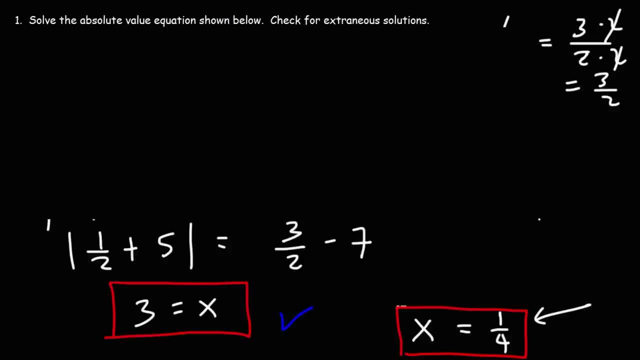 Now 1, half plus 5.. So let's get common denominators. We can multiply 5, or 5 over 1, by 2 over 2. And this will give us 10 over 2.. Now we can do the same thing with negative 7.. 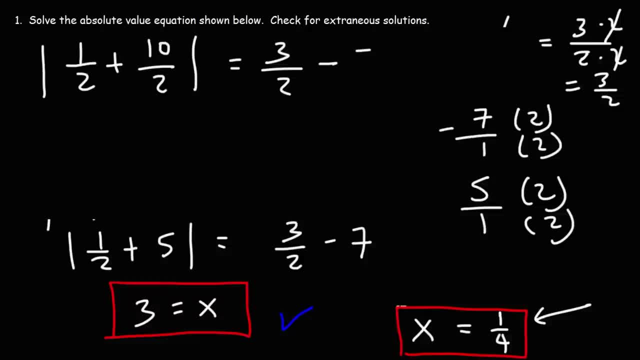 If we multiply it by 2 over 2, this becomes negative 14 over 2.. So now that we have the same denom denominator, we can add the numerators of the 2 fractions. 1 plus 10 is 11.. 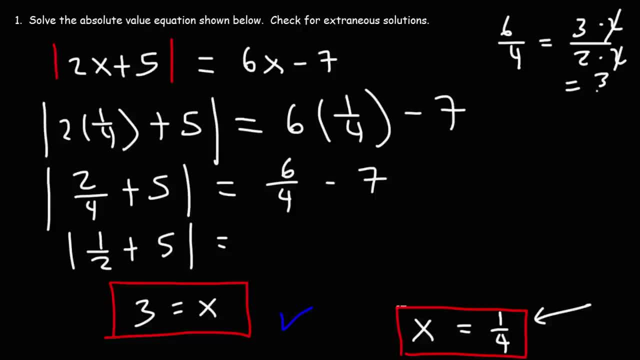 times 2.. Canceling the 2, we can reduce that to 3 over 2.. Now 1 half plus 5,. so let's get common denominators. We can multiply 5, or 5 over 1, by 2 over 2, and this will give us 10 over 2.. Now we can do the same thing with negative. 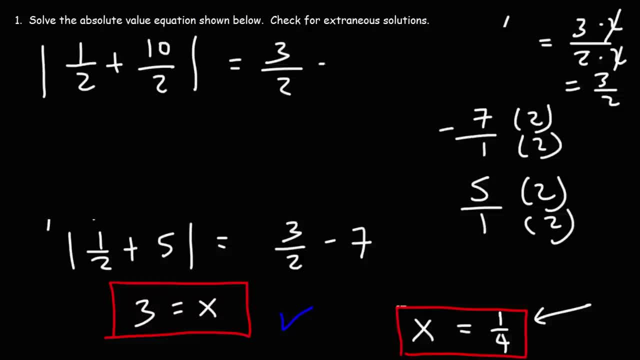 7. If we multiply by 2 over 2, this becomes negative 14 over 2.. So now that we have this same denominator, we can add the numerators of the two fractions. 1 plus 10 is 11,, so 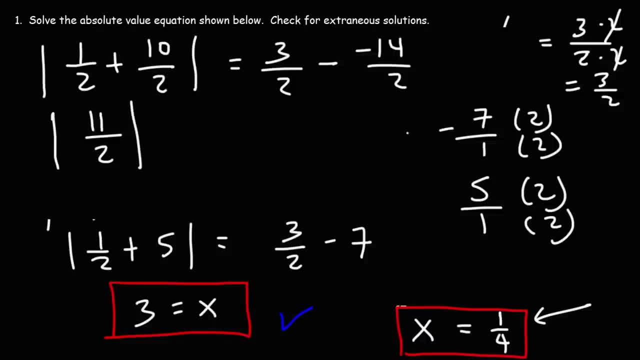 we get 11 over 2.. By the way, I have two negatives here. We should only have one negative, like we had here Now. 3 minus 14 is negative 11.. What is the absolute value of positive 11? 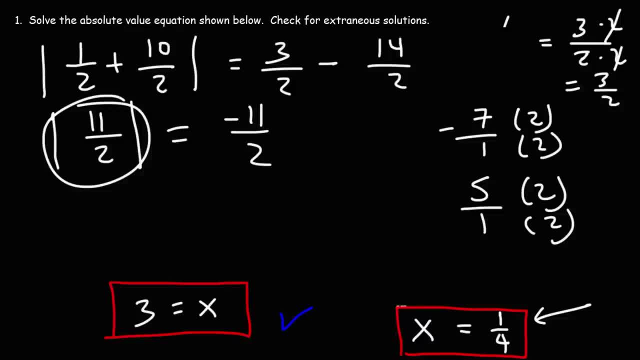 over 2?? Well, the absolute value of any number will always give you a positive result, unless you're taking the absolute value of 0,, of course, The absolute value of 11 over 2 is positive 11 over 2, and this does not equal negative 11 over 2.. So, therefore, because 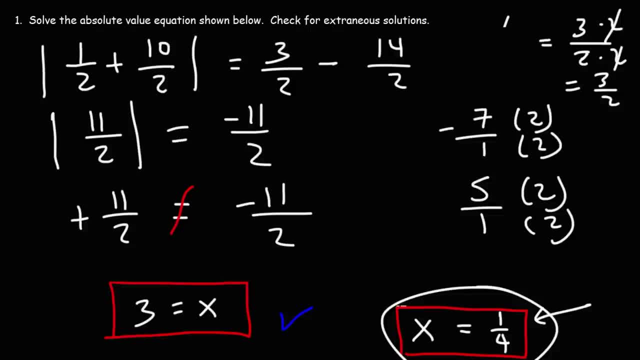 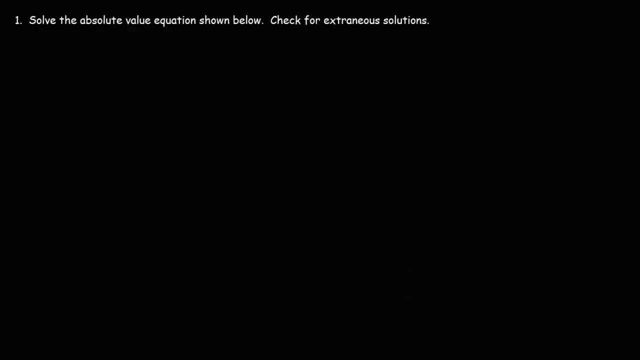 this solution here doesn't work. in the original equation this is the extraneous solution. So that's how you can find the extraneous solution when solving absolute value equations. Now let's go ahead and try another example. Let's say we have the 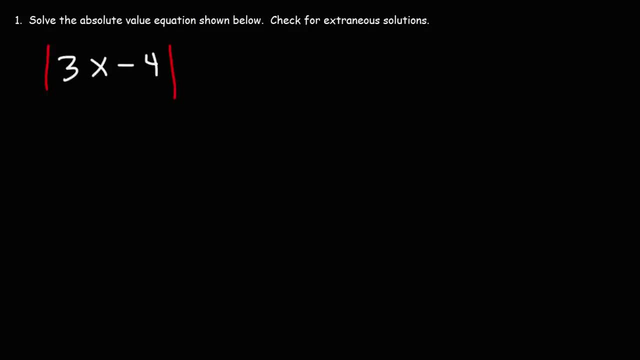 absolute value of 3x minus 4, and let's set that equal to 2x minus 6.. Go ahead and set it to 0,. okay, Go ahead and solve this one. So let's begin by writing two equations. 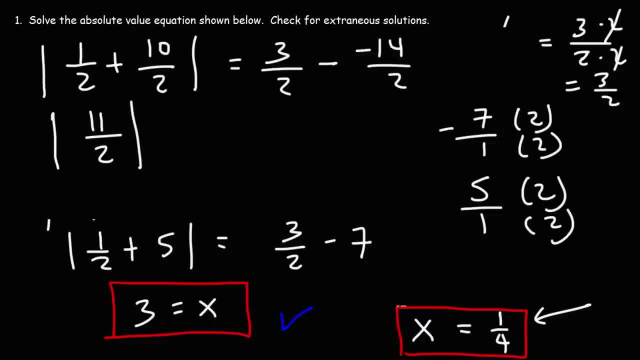 So we get 11 over 2.. By the way, I have 2 negatives here. We should only have 1 negative Now. 3 minus 14 is negative 11.. What is negative? 14 over 2?? ketos mean 3.. 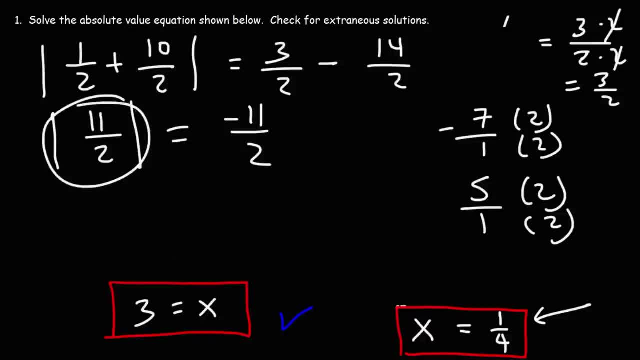 equation, the absolute value of positive 11 over 2, the absolute value of any number- will always give you a positive result, unless you're taking the absolute value of 0, of course. the absolute value of 11 over 2 is positive 11 over 2 and this does not. 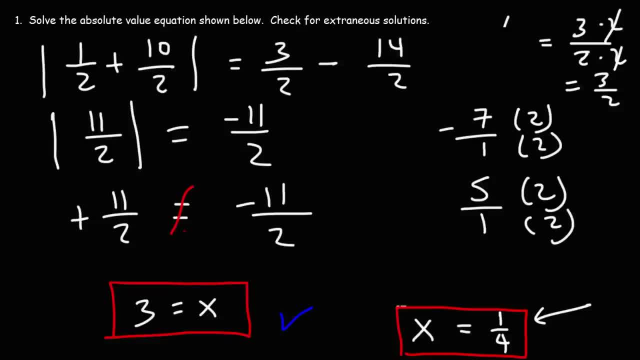 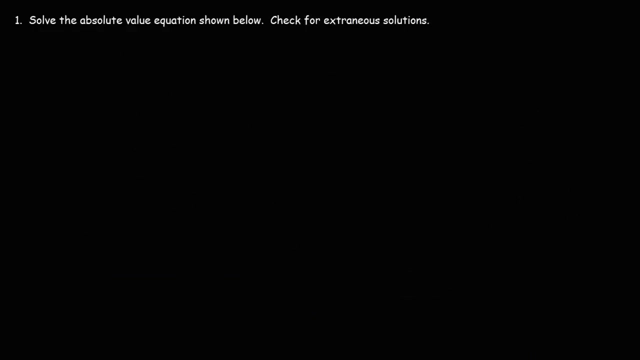 equal negative 11 over 2. so therefore, because this solution here doesn't work in the original equation, this is the extraneous solution. so that's how you could find the extraneous solution when solving absolute value equations. now let's go ahead and try another example. 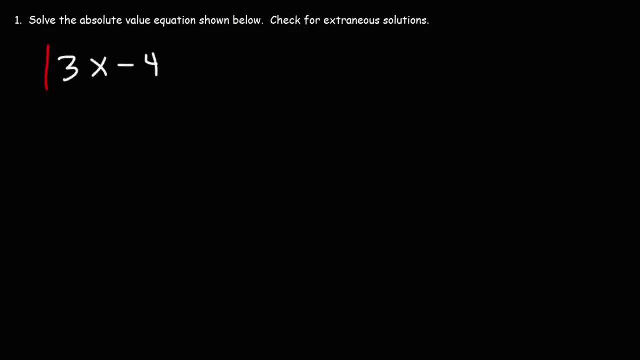 let's say we have the absolute value of 3x minus 4 and let's set that equal to 0, 2x minus 6. go ahead and solve this one. so let's begin by writing two equations: 3x minus 4 is going to equal to positive. 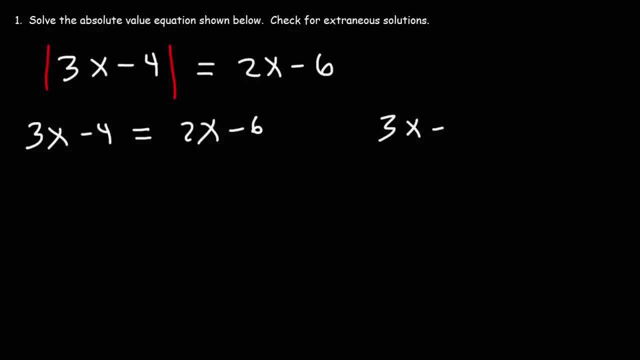 2x minus 6, and also 3x minus 4. that's going to be equal to negative times 2x minus 6. so let's start with the first one. let's subtract 2x by both sides and let's add 4 to both sides of the equation. 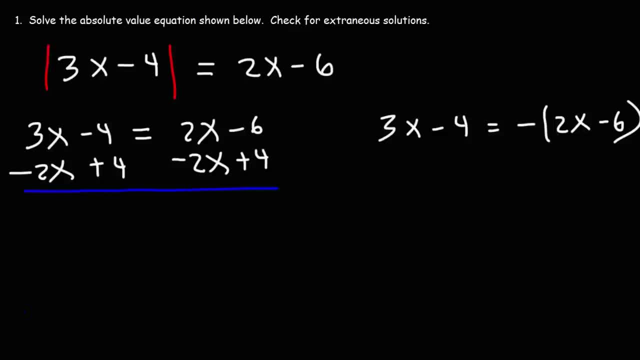 doing it this way, we'll put all of the x variables on one side and then we'll have a number on the other side. 3x minus 2x is 1x, which we can write it as x negative. 6 plus 4 is negative 2. so this is our first solution: x is equal to negative 2. 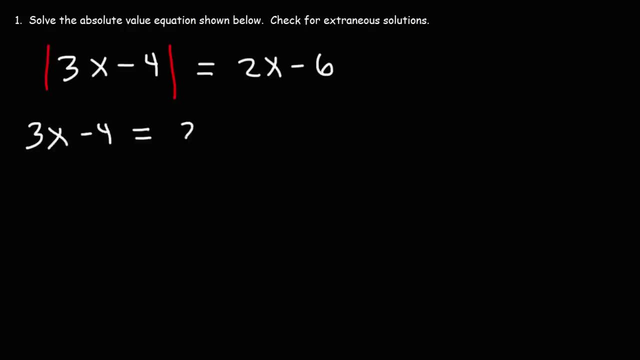 3x minus 4 is going to equal to positive 2x minus 6, and also 3x minus 4,, that's going to be equal to negative times 2x minus 6.. So let's start with the first one. 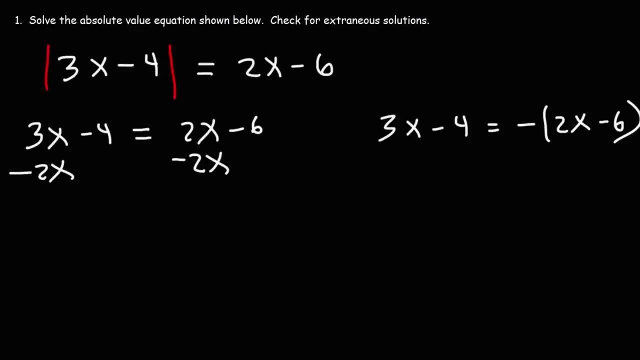 Let's subtract 2x by both sides And let's add 4 to both sides of the equation. Doing it this way, we'll put all of the x variables on one side and then we'll have a number on the other side. 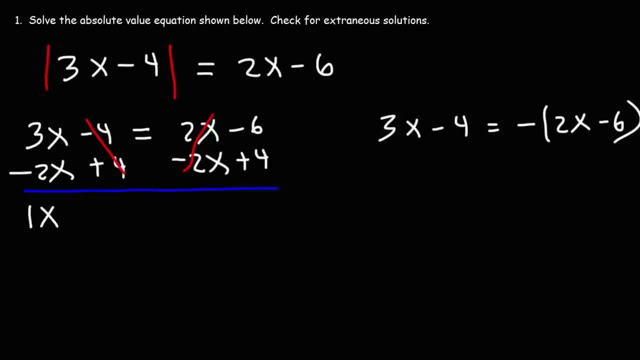 3x minus 2x is 1x, which we can write it as x Negative. 6 plus 4 is negative 2.. So this is our first solution: x is equal to negative 2.. Now let's focus on the other equation. 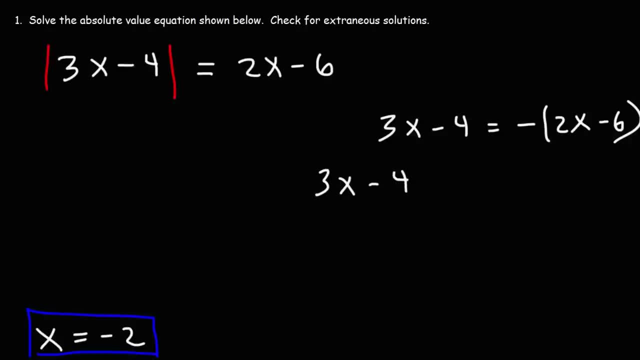 Let's begin by distributing the negative sign, So we're going to have negative 2x and positive 6.. Now, instead of subtracting both sides by 3x, which will give us negative 5x on the right side, Let's add 2x on both sides, so we'll get positive 5x on the left side. 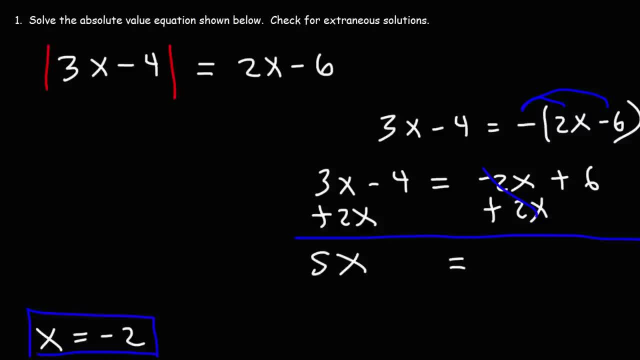 Those two will cancel. Now, instead of subtracting both sides by 6, which will leave a 0 on the right side, let's add 4 to both sides. 6 plus 4 is 10.. Now let's divide both sides by 5.. 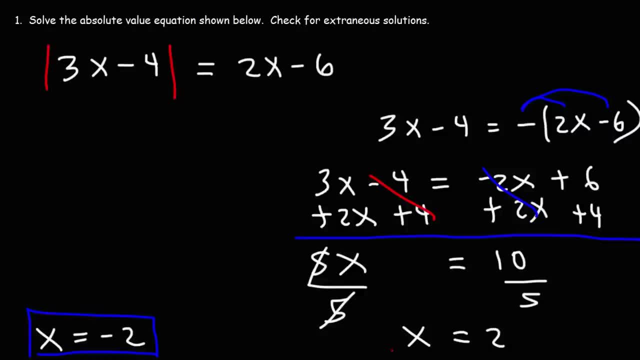 10.. 10 divided by 5 is 2.. So the other answer is: x is equal to positive 2.. So which one of these two solutions is the extraneous solution? What would you say? Is it negative 2 or is it positive 2?? 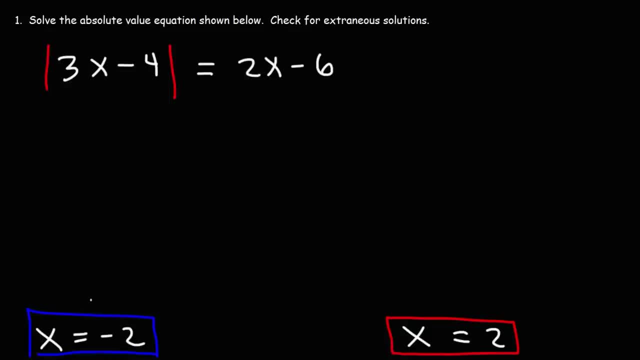 Well, we need to plug it into the original equation to find the answer. So let's begin by plugging in negative 2.. 3 times negative 2 is negative 6.. 2 times negative 2 is negative 4.. Negative 6 minus 4 is negative 10.. 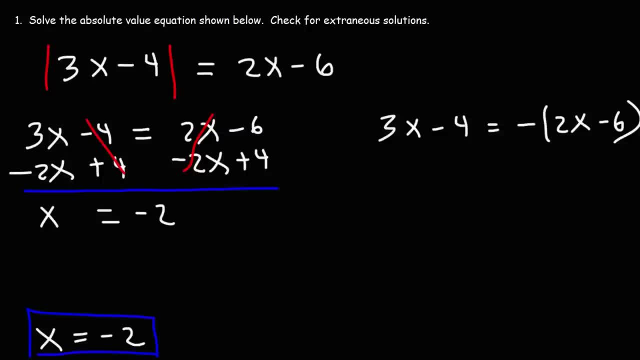 negative two. Now let's focus on the other equation. Let's begin by distributing the negative sign. So we're going to have negative 2x and positive 6.. Now, instead of subtracting both sides by 3x, which will give us negative 5x on the right side, let's add 2x on both sides. 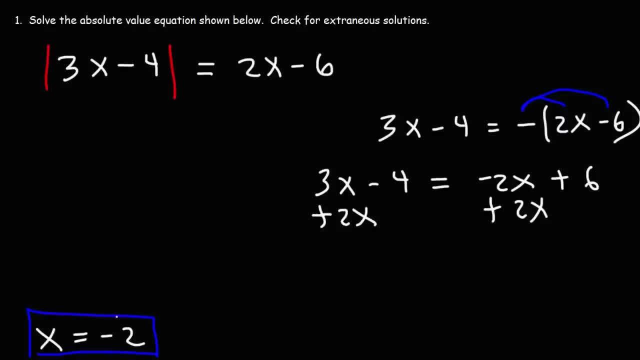 so we'll get positive 5x on the left side. Those two will cancel. Now, instead of subtracting both sides by 6, which will leave a 0 on the right side, let's add 4 to both sides. 6 plus 4 is 10.. 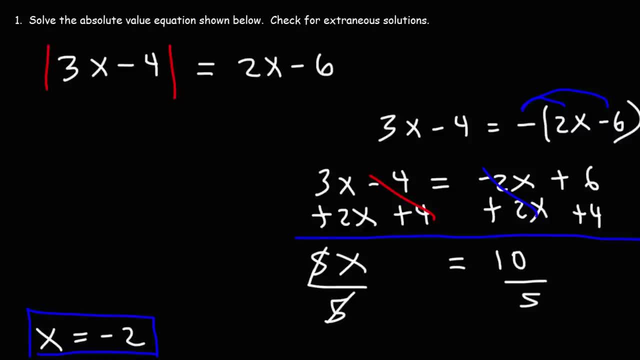 Now let's divide both sides by 5.. 10 divided by 5 is 2.. So the other answer is: x is equal to positive 2.. So which one of these two solutions is the extraneous solution? What would you say? 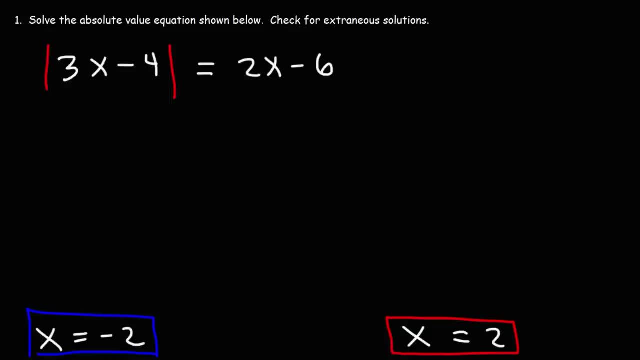 Is it negative 2 or is it positive 2?? Well, we need to plug it into the original equation to find the answer. So let's begin by plugging in negative 2.. 3 times negative 2 is negative. 6.. 2 times negative 2 is negative. 4. Negative 6 minus 4 is negative. 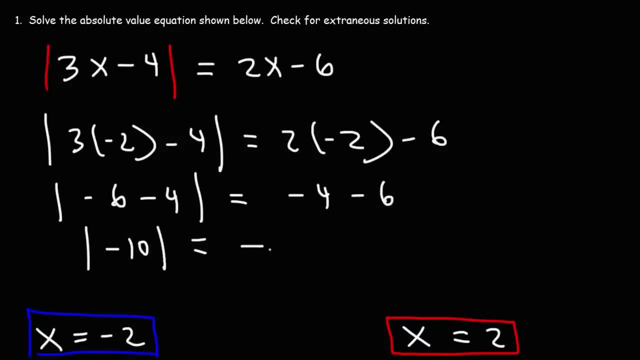 10.. And the same is true for negative 4 minus 6.. That also equals negative 10.. Now, the absolute value of negative 10 is positive 10.. And positive 10 is the absolute value of negative 10.. So we're. 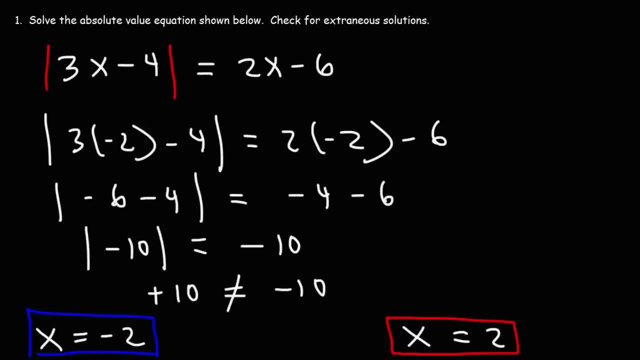 going to have. negative 10 does not equal negative 10.. So this here, because it doesn't work for the original equation. this is the extraneous solution. Now let's check the other answer as well. So we're going to have 3 times 2 minus 4. And the absolute value.